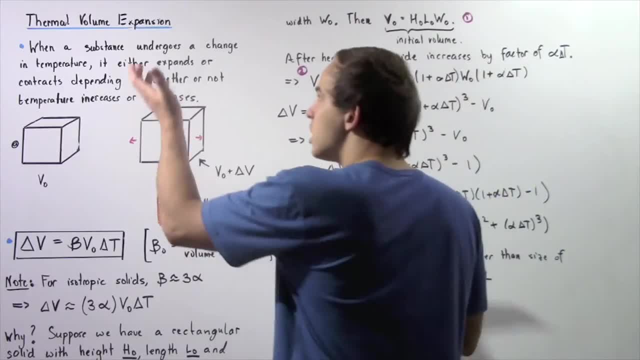 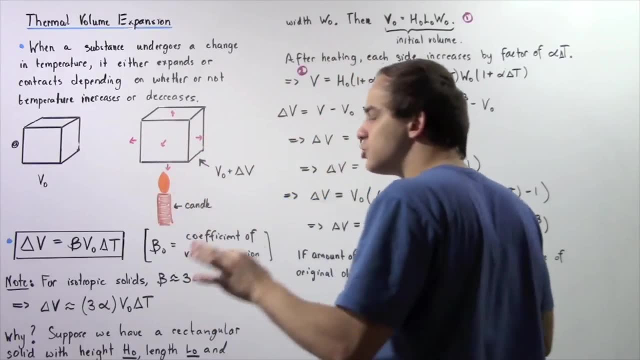 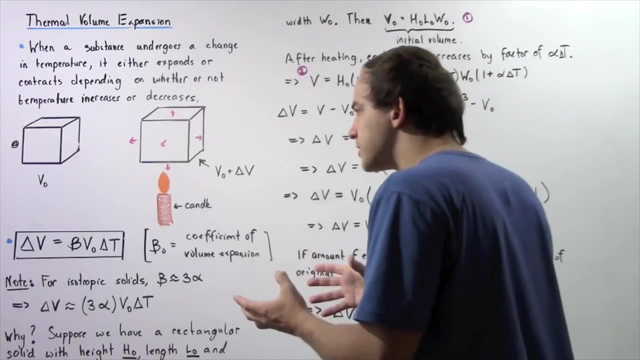 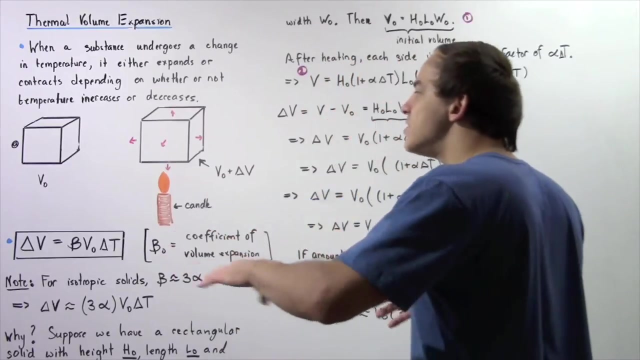 the object will expand out of the solid object. So after some time the object will expand outward in all possible directions and this is known as thermal volume expansion. So the reason the object expands is because the individual atoms and molecules inside our solid object will vibrate more vigorously and that means the distance between any two adjacent atoms or molecules will increase and that collectively will increase the entire volume of our object. 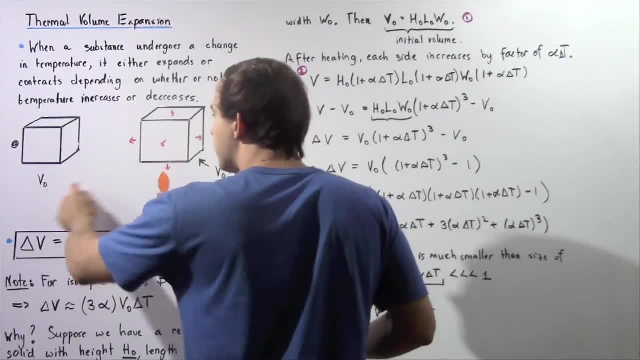 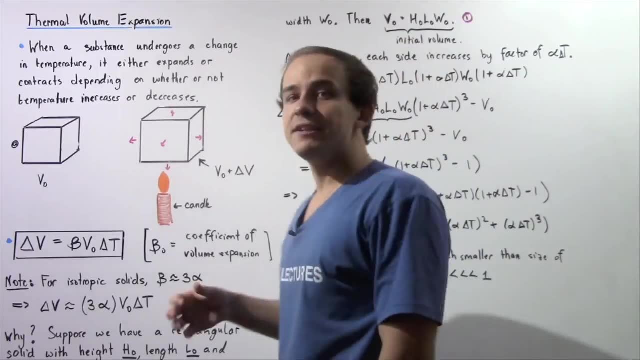 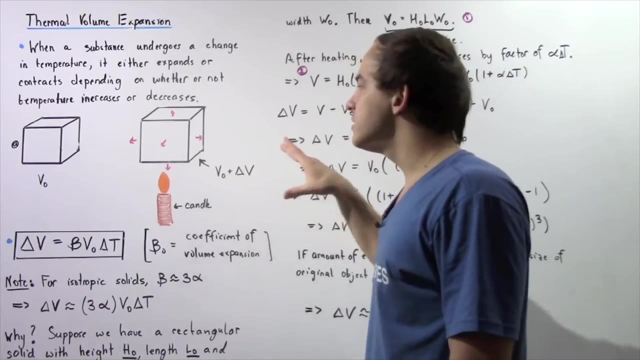 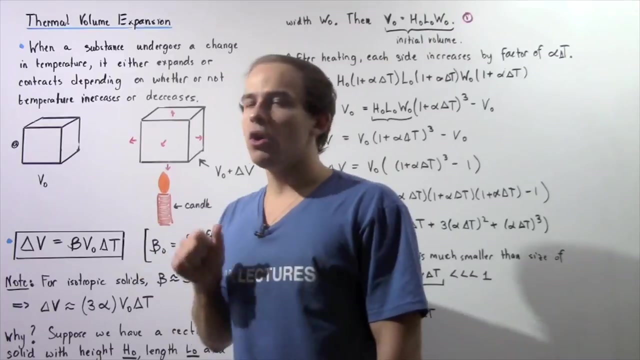 So if the initial volume of the object is given by V0, and the object expands by a volume given by delta V, then the final volume of our object is given by V0 plus delta V. Now, in the same exact way that we were able to develop a formula for thermal linear expansion of objects, we also have a formula for thermal volume expansion of objects given by the formula for thermal linear expansion of objects. 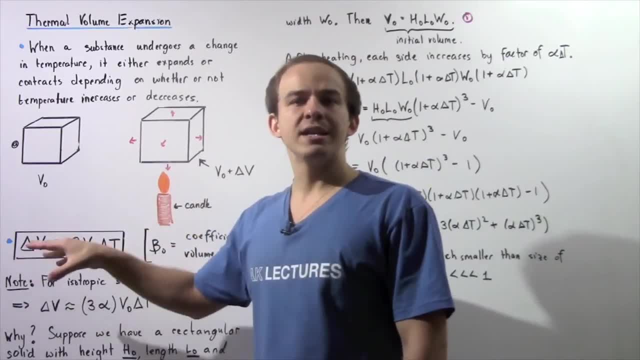 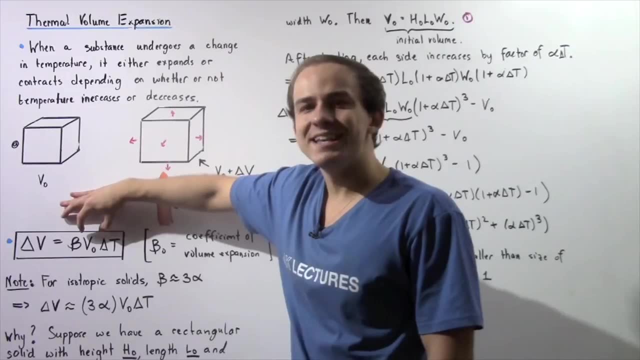 So the inductive jungle donation of the delta V is the following equation: So weус, as we read in the equation box, will be given by delta Vивается, which is the coefficient stress Now, if N, of the greatest. 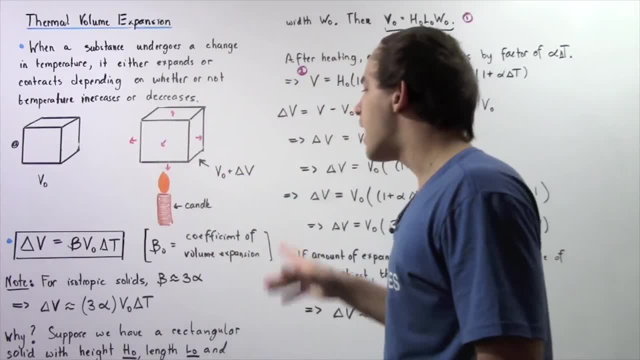 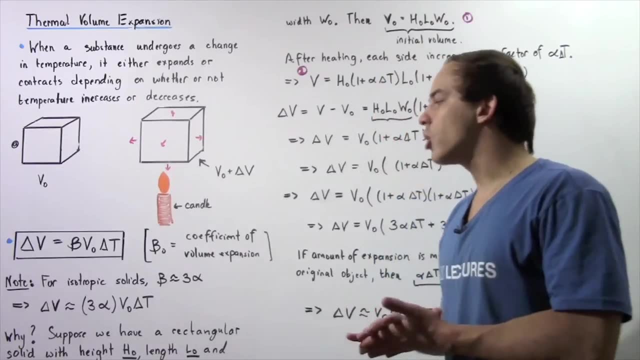 caring requests to be minus 15 needed. So in other words, when the overall temperature falls for T minus 16, the constant will get decrease. so the total amount of balance which land on the distance between tolerated components X and taking the metros for travelers, When the coefficient stress getsoto the total 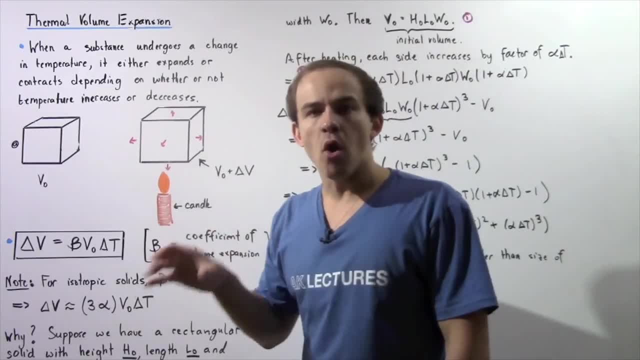 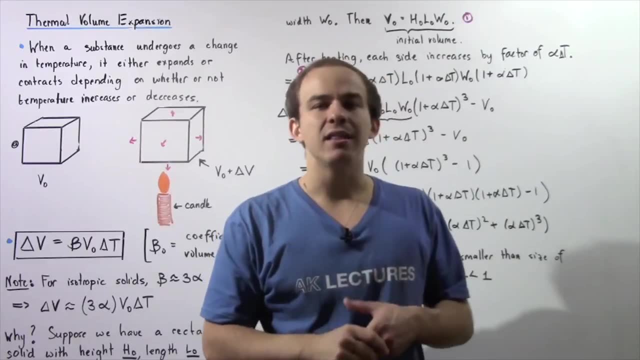 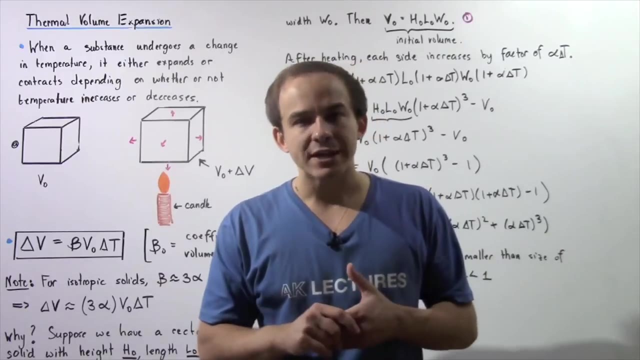 component Y is the most satisfying because the am Hera was given by delta Vxt at the value much smaller than v naught. So let's suppose that we are talking about isotropic solids. Isotropic solids are those solids that have the same exact properties in all different directions. 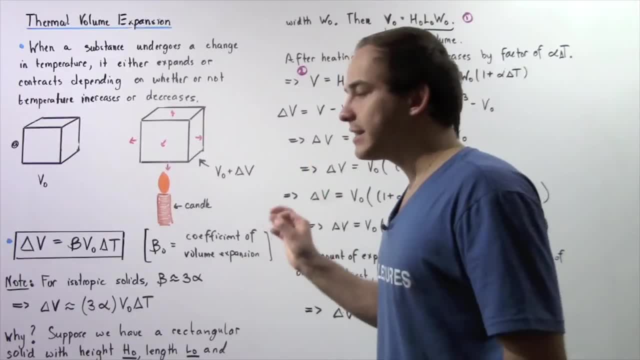 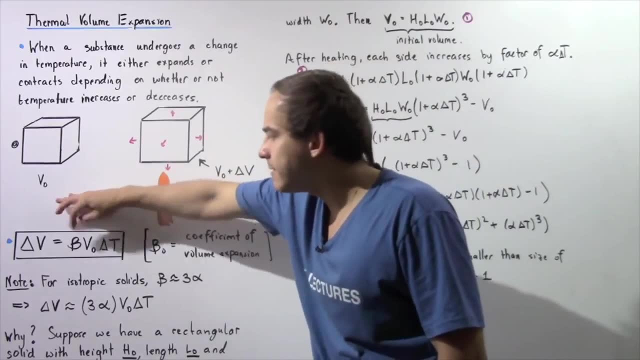 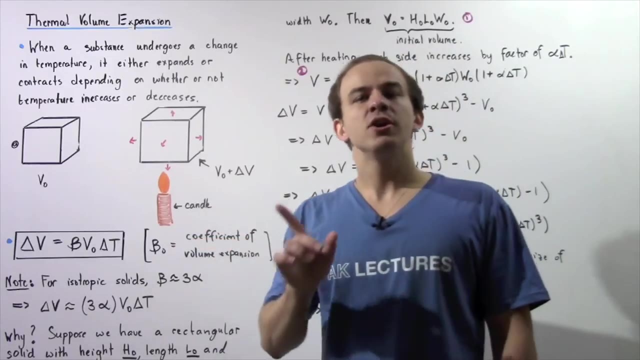 such as density. Now, if our object, if our solid object, is in fact isotropic, that means we can approximate the beta value to be approximately equal to three times the alpha, And alpha is simply the coefficient of linear expansion that we spoke about in the previous lecture. 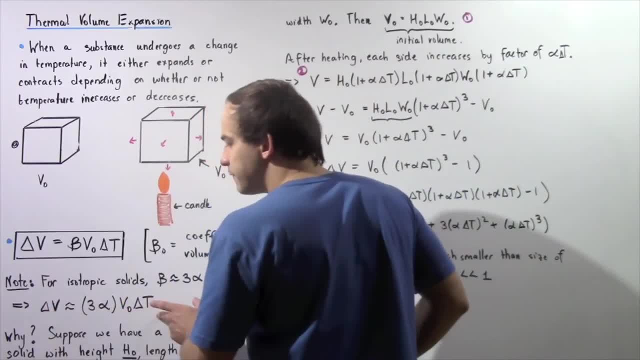 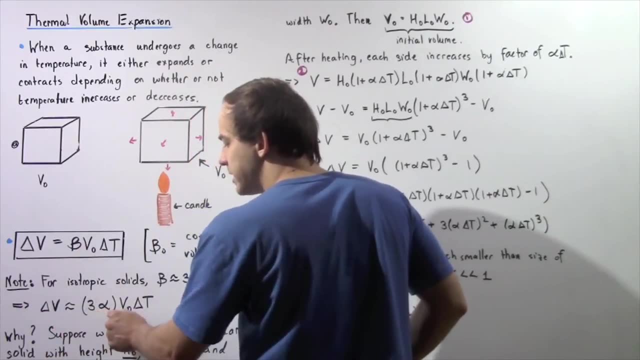 From this approximation we have the following formula: The change in volume is approximately equal to. we replace our beta with three alpha. So three alpha multiplied by v, naught multiplied by three alpha. So we have the following formula. We have the following formula. We have the: 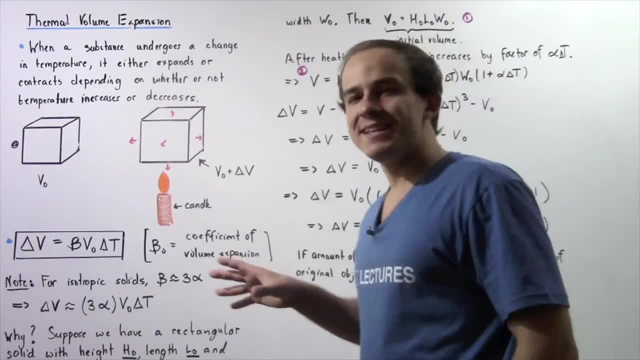 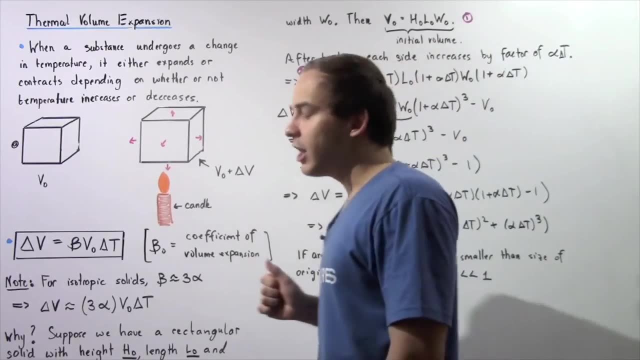 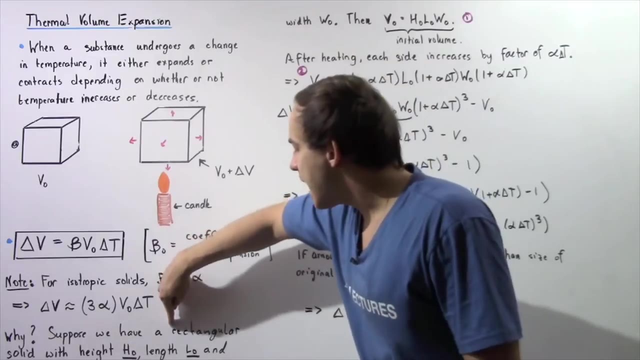 change in temperature. So why is this true? Well, we're going to prove this in the following several steps, But first let's make the following assumption: Suppose that we are dealing with an isotropic solid, And suppose that we are dealing with a solid that is a rectangle that has a height. 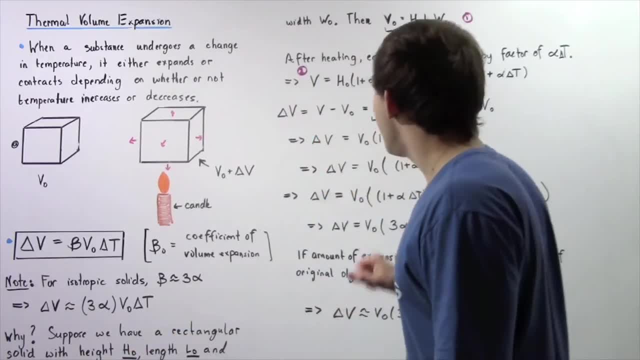 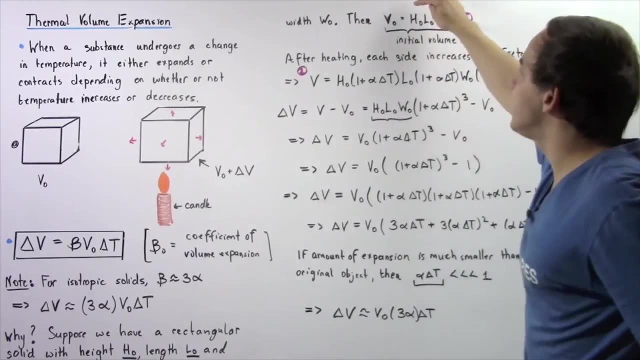 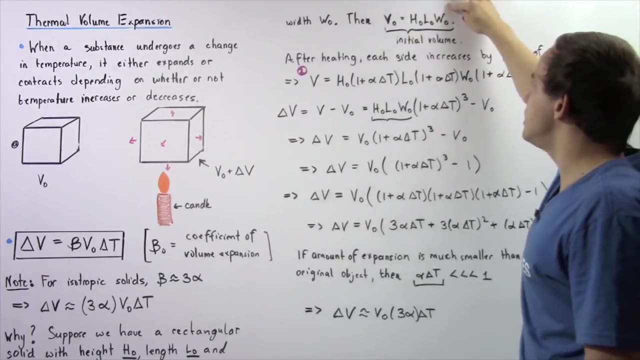 given by h naught, a length given by l naught and a width given by w naught. Using these parameters, we can calculate the initial volume- v naught- of our solid rectangular object by simply taking the product of these three lengths, So length, the height and the width. 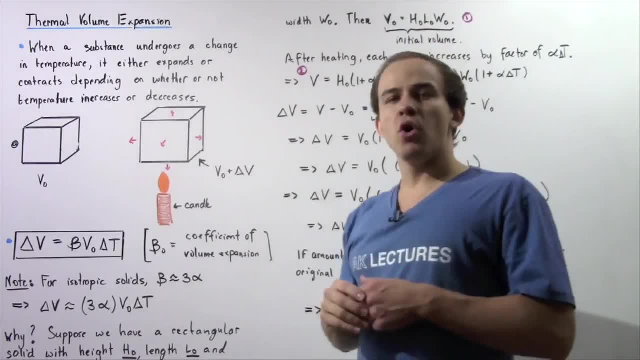 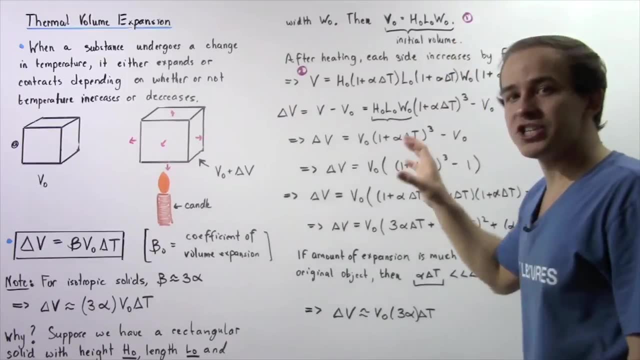 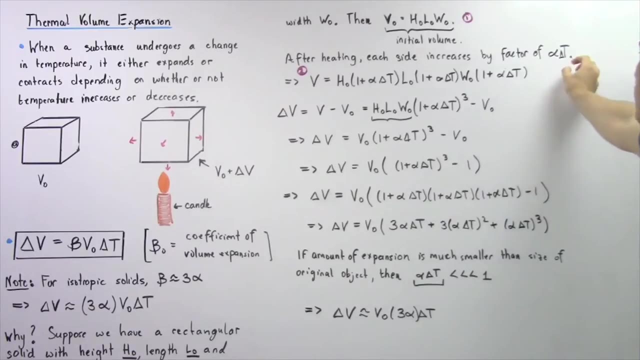 gives us the initial volume. Now let's suppose we take a heat source, For example our candle. we heat the object And after heating, each side of our rectangular object will increase by a factor of our alpha multiplied by delta t. This is what we spoke about in the previous lecture. 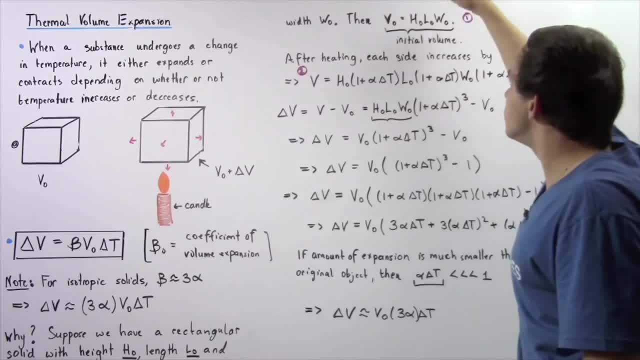 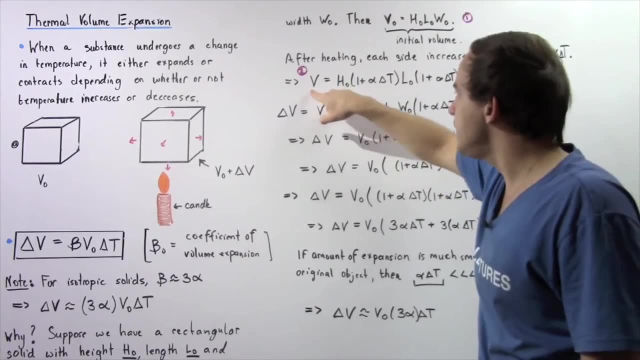 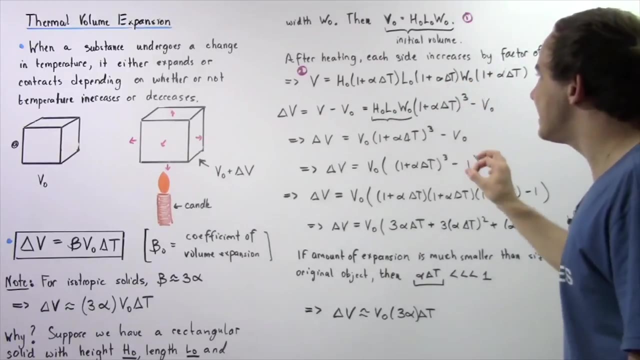 So that means every single one of these sides will increase by that factor. So we have: the final volume given by v is equal to h naught multiplied by l naught, multiplied by w naught, And every single side is increased by delta t. So we have the final volume given by v is equal to h naught. 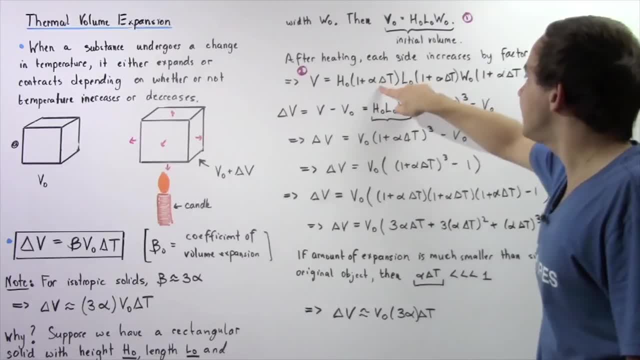 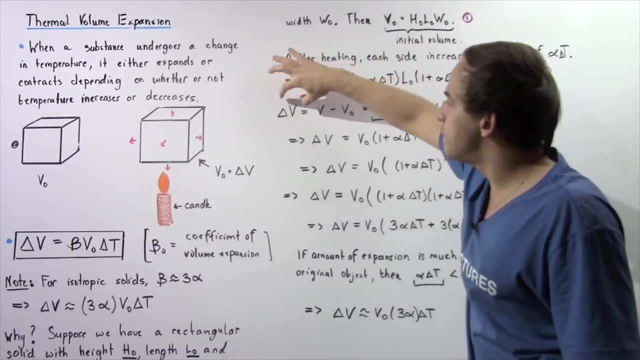 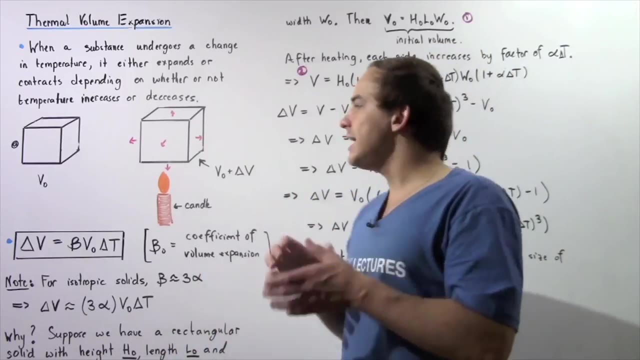 multiplied by delta t. So let's call this equation two. Let's call this equation one. Then, if we want to find the change in volume, we simply take the final volume after heating and subtract the initial volume. So equation two, or equation one minus equation two, We have 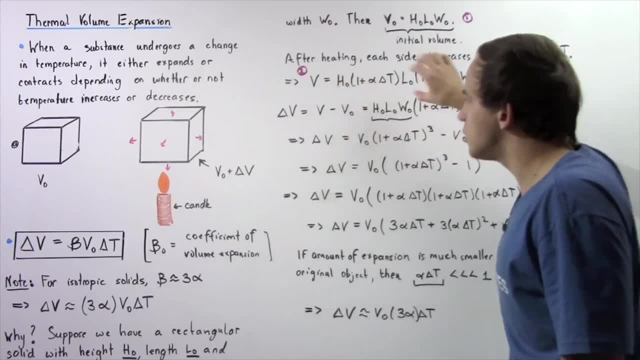 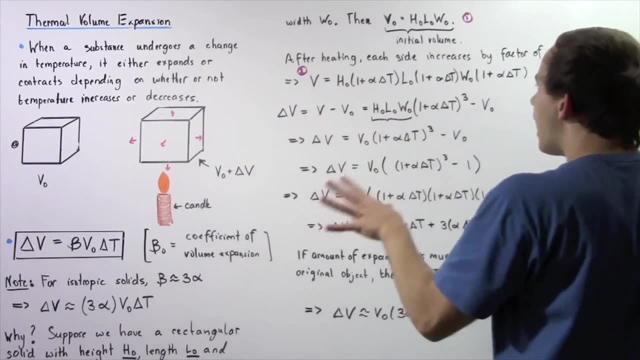 v minus v naught. So we're subtracting v initial from v final, So we have v minus v naught And this is equal to well, we have this entire equation. So let's combine a few terms, Let's. 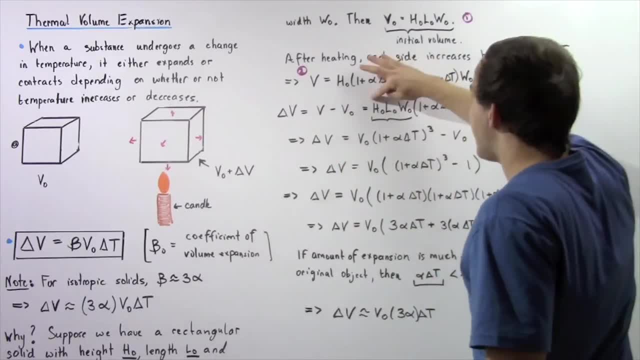 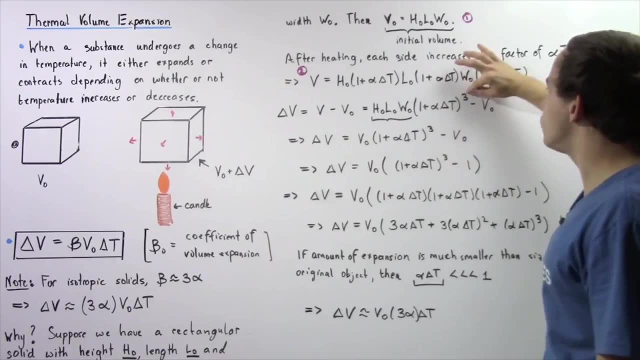 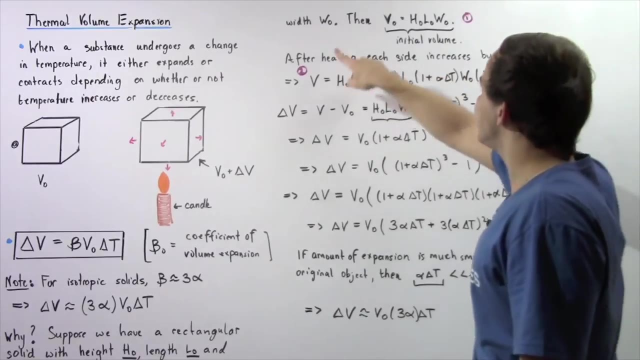 combine these three identical terms And we get h naught, l naught, w naught, multiplied by one, plus alpha multiplied by delta t, And we raise it to the power of three, because we have three identical terms. And then we subtract equation one. So we subtract v naught. Now notice: 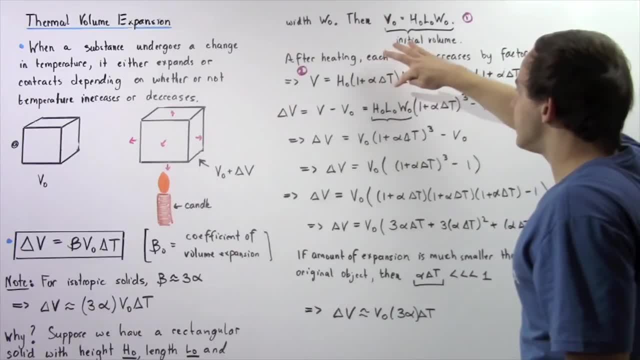 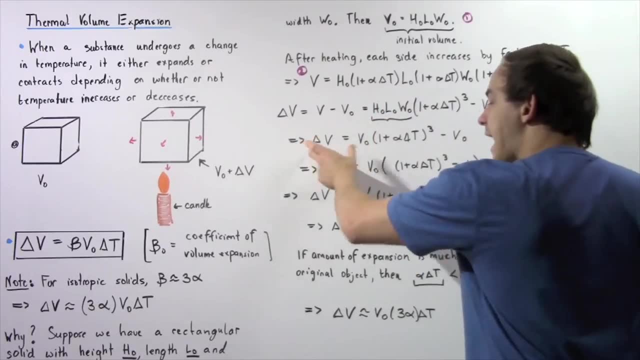 according to equation, one h naught times l, naught times w naught is simply v naught. So we replace this with v naught And we have delta v. our change in volume after heating is equal to v naught. 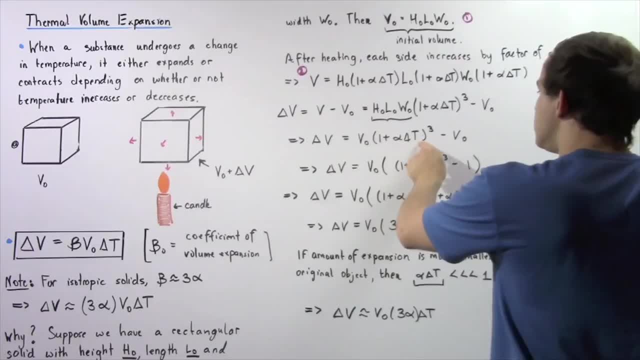 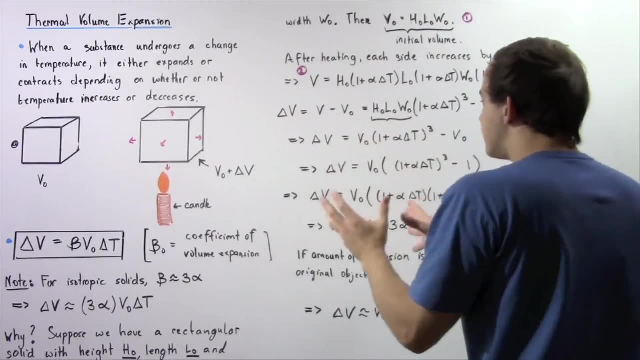 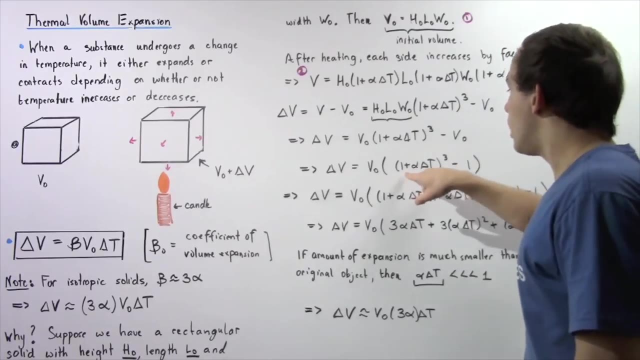 multiplied by one plus alpha times. delta t to the third power minus v naught. So notice, v naught appears on both terms. So we can take that out and we get the following result: Delta v is equal to v naught multiplied by one plus alpha times. delta t to the third power minus one. Now if we 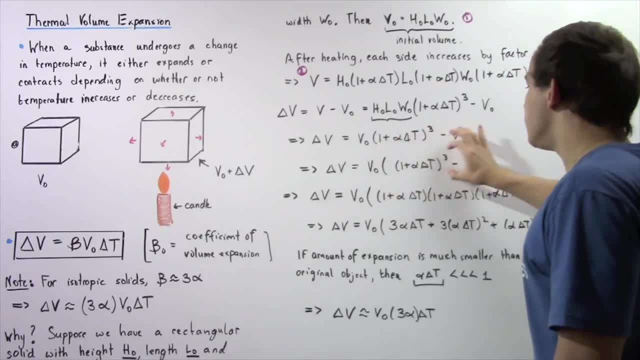 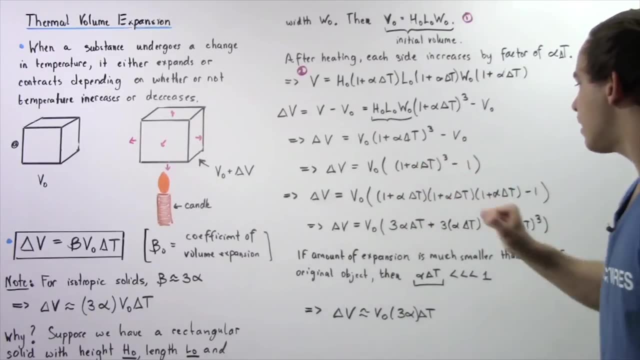 expand the following equation and multiply it out. we get the following result. So we expand it as shown, We multiply it, We add things out, Notice the ones will cancel And we're left with the following result: Delta v is equal to v naught multiplied by three times alpha times delta t. 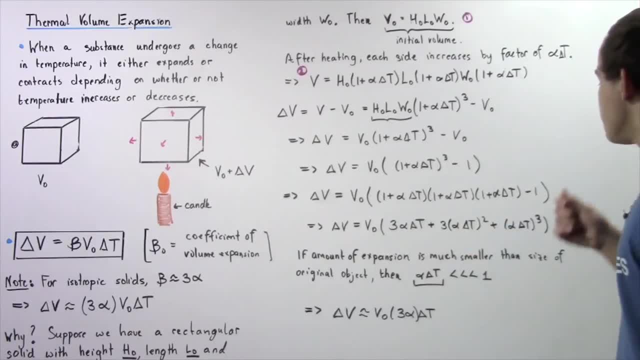 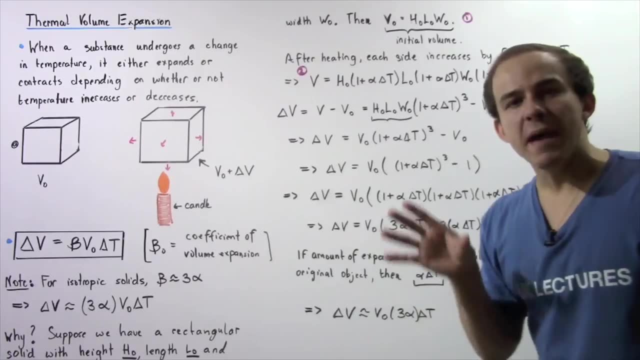 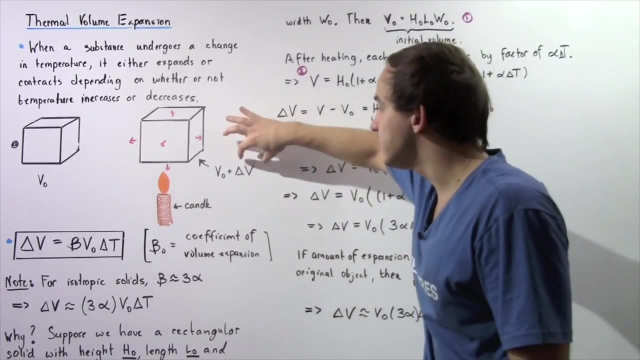 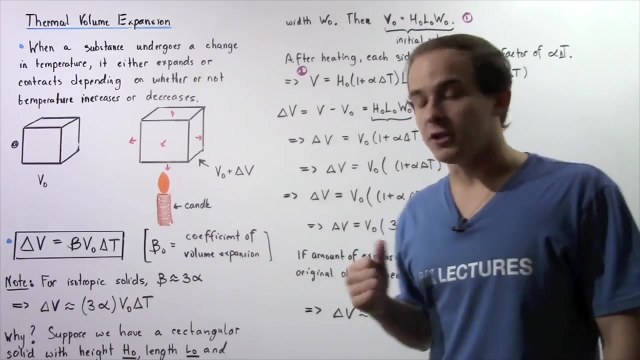 plus three times the square of alpha times, delta t plus the cube of delta times change in t. Now, if the amount of expansion is much smaller than the size of the original object, if the delta t is smaller than v naught, then this term becomes very, very small, because our change in t multiplied. 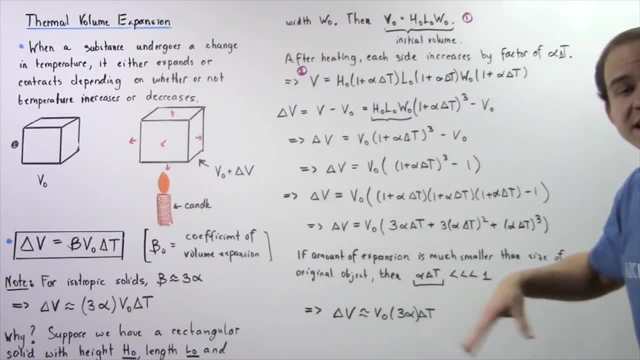 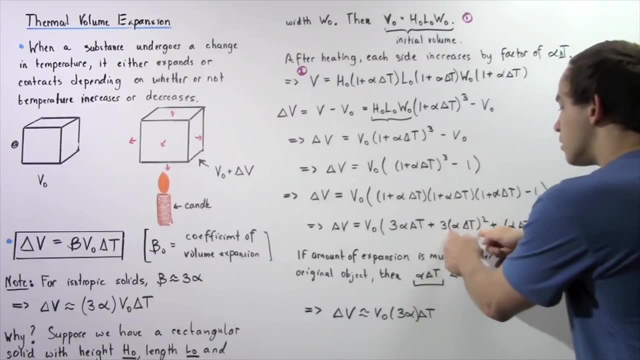 by a very small value of v naught is very, very small. So we have a very small value of v naught. The value of delta gives us a number that is much smaller than 1.. And that means a number that is much smaller than 1 to the square is a small number.